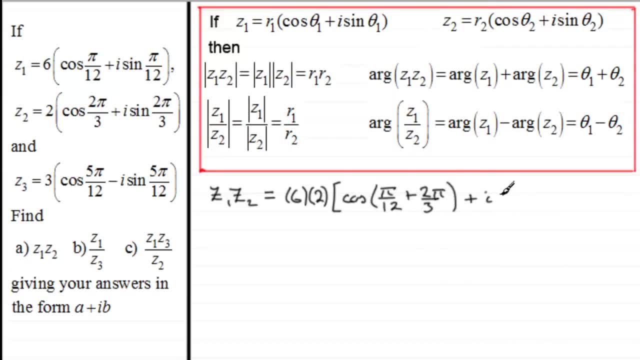 And we've also got plus i sine of that arg as well. So that's going to be again the same angle: pi upon 12 plus 2 thirds pi. Okay, so we'll just finish that bracket off there. Now, if we tidy this up, we've got 6 times 2, which is 12, and then we've got that. this is: 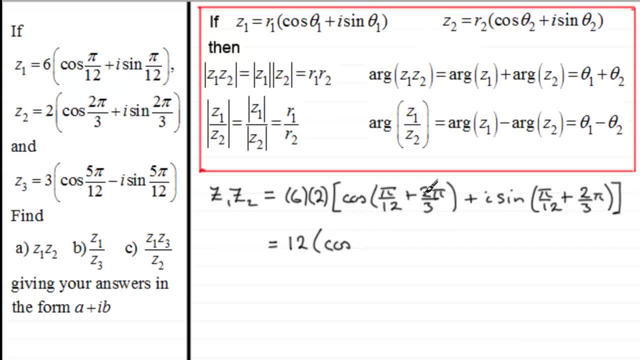 all multiplied by the cosine of pi upon 12 plus 2 thirds pi, That comes to 3 quarters pi. So 3 pi over 4 or 3 quarters pi there And the same here, only it's going to be plus i sine of 3 quarters pi. 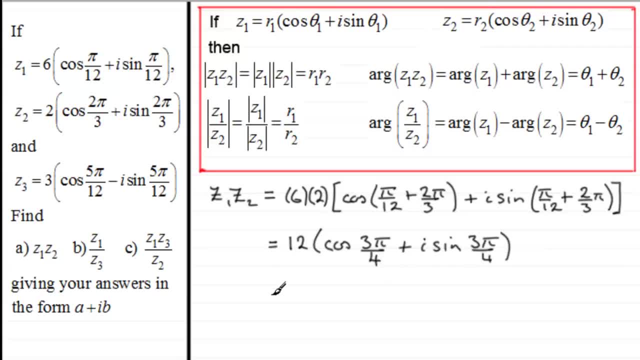 Now, don't forget, this angle here is in radians. okay, So if you work this out, the cosine of 3 pi upon 4 is exactly minus root 2 over 2.. And then here, the sine of 3 pi upon 4 is plus root 2 over 2.. 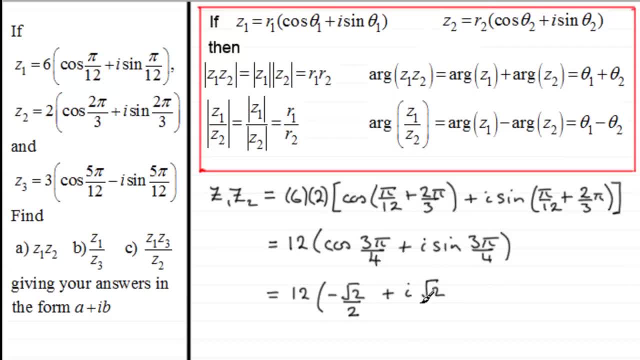 So you've got plus i times 2.. Plus i times root 2 over 2.. So that when we multiply through by 12 we end up with minus 6 root 2 and then plus i times 6 root 2.. Okay, so hopefully that gives you an idea on part a then. 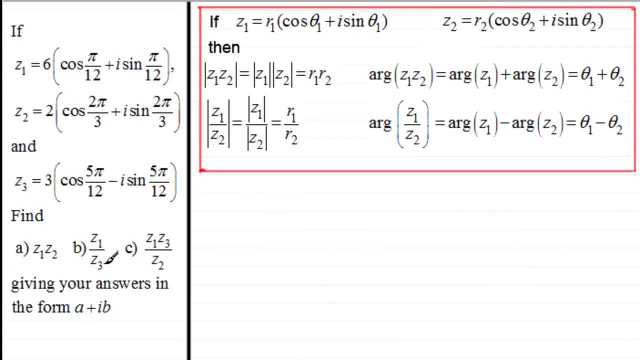 Now for part b, we've got to work out z1 divided by z3. And for this I picked this one, because you'll find that z3 has got a negative here, And what I've given you up here are the results when we have a plus. okay. 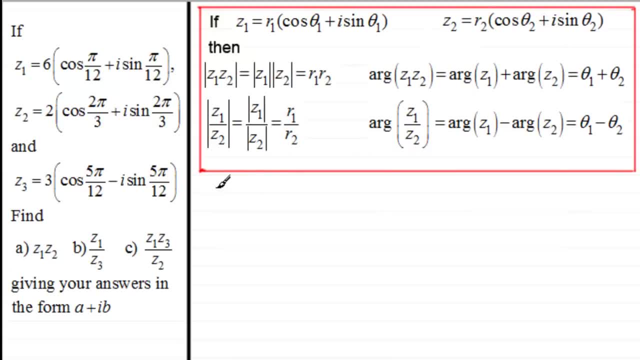 So this is the point behind this question. We've got to modify z3 first of all. Now we know that z3 then is equal to 3 multiplied by the cosine. Okay, We'll just put this in brackets: Cosine of 5 pi upon 12 minus i sine of 5 pi upon 12.. 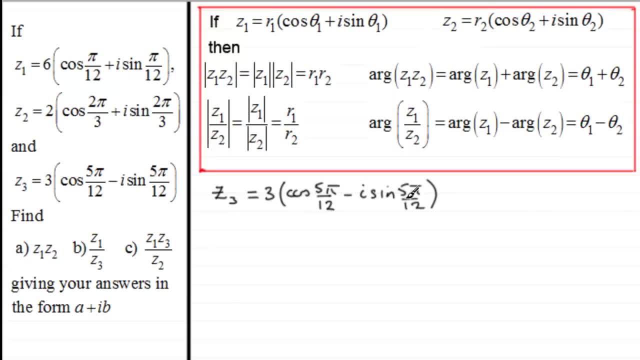 Now we need to change this, then, and we should be familiar with the result that when we have a negative here, this is exactly the same as saying 3 times the cosine, okay, of the negative of this angle minus 5 pi upon 12.. 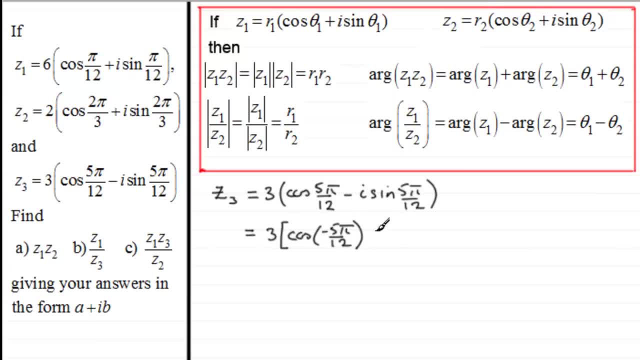 Let's say, a result that we should be familiar. if not, just check out my tutorials on the mod arg form for this, okay. And then we've got plus. and then for this one it's plus i sine of the negative, minus 5 pi over 12, okay. 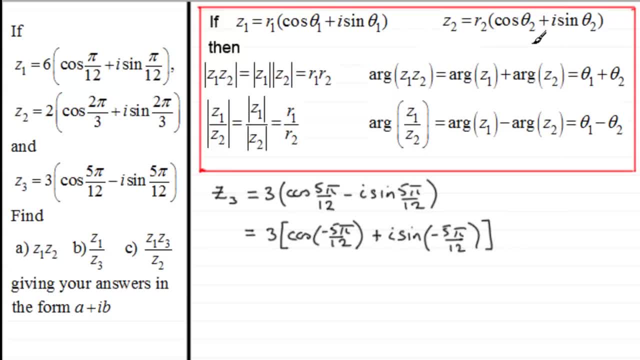 So we've now got this in the right format, and when it comes to working out what z1 divided by z3 is, if we were to put this in mod arg form first of all, then the modulus is going to be the mod of z1 divided by the mod of z3. 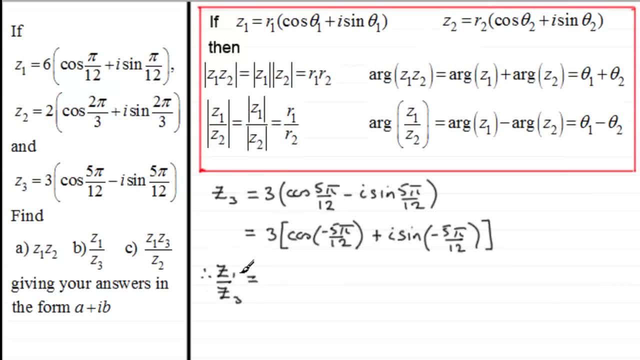 This result up here, And so the modulus of z1 is 6 and the modulus of z3 is 3.. So we'll just write that as 6 over 3 for the moment, And then that is multiplied by the cosine of the arg for z1.. 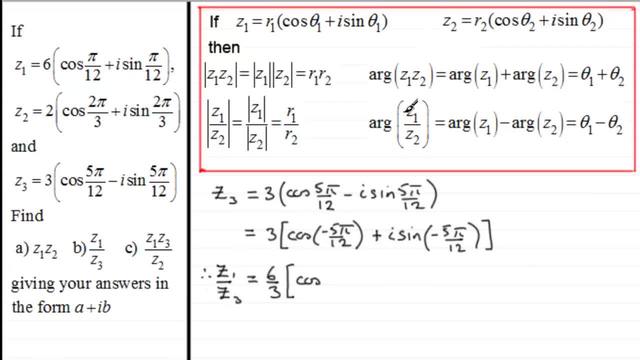 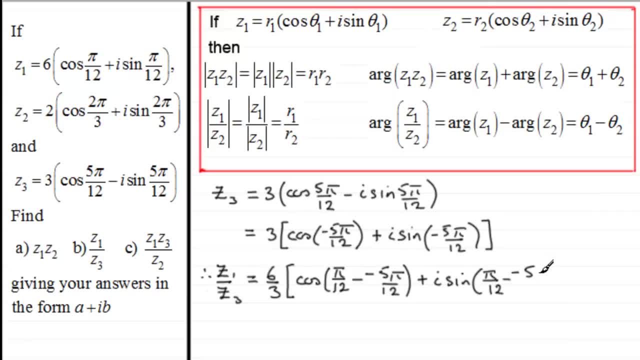 Pi upon 12 minus minus 5 pi upon 12.. And what does this give us? Well, 6 divided by 3, then here is clearly 2, and then we've got the cosine of pi upon 12 minus 5, pi upon 12.. 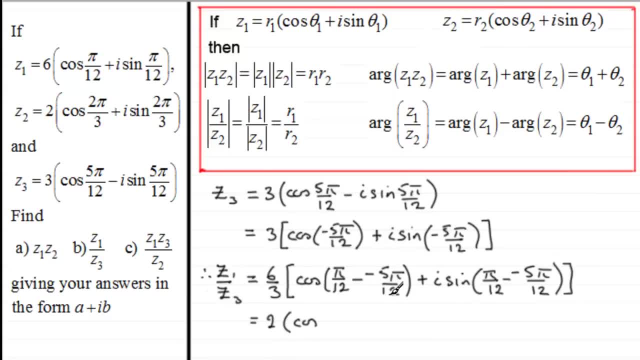 And then we've got the cosine of pi upon 12 minus 5 pi upon 12.. And then we've got the cosine of pi upon 12 minus 5 pi upon 12.. Plus 5 pi upon 12, which is 6 pi upon 12 or pi upon 2.. 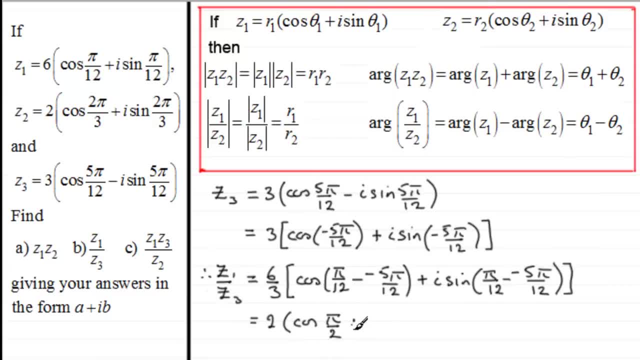 So we've got the cosine of pi upon 2 plus, and then the same again, only this time with sine i, sine pi upon 2.. And the cosine of pi upon 2 radians is 0.. Sine of pi upon 2 radians is 1.. 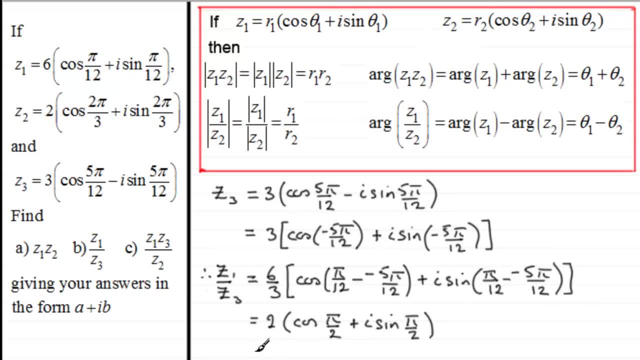 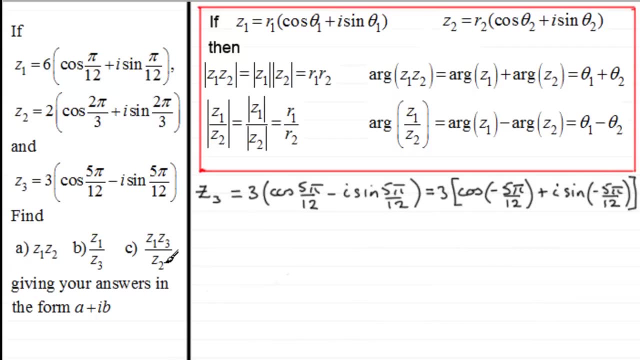 So all you end up with is that this equals to I. okay now in part C, for Z 1 times Z 3 divided by Z 2. I showed you that in Part B- Z 3- because it was in the wrong format. it's got a minus here. we had to. 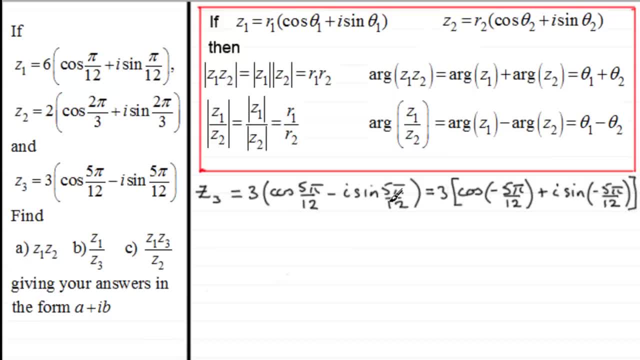 change it to a plus. I applied the rule that this was the same as the cosine of minus 5 pi upon 12, plus I sine minus 5 pi upon 12, a well-known result which, if you're not familiar with you, can always check out on my website. okay, just by. 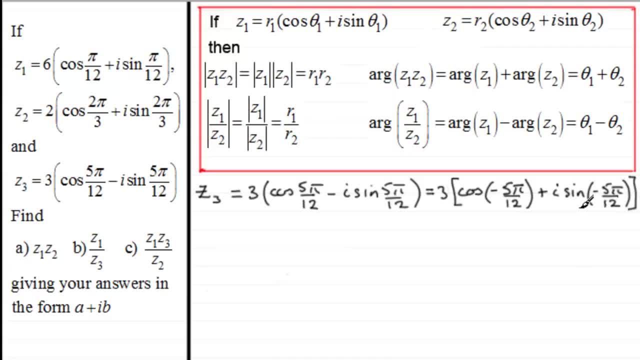 looking on the mod ARC form of a complex number. well, with that result we can now work out then: Z 1 times Z 3 over Z 2, so we're going to have then, therefore, Z 1 times Z, Z 3, all divided by Z 2. well, first of all, to put this thing in mod ARC form, we 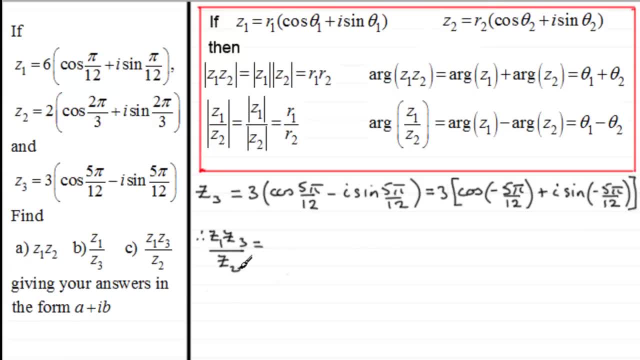 need the mod of Z 1 times Z 3 over Z 2. so the mod of Z 1 times Z 3 is going to be the modulus by this result of the product of the individual module I. so that's going to be 6 times 3. okay, 6 times. 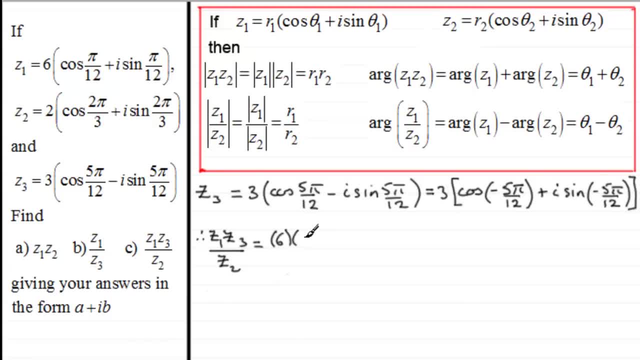 3, then for the first part, and then this is divided by the modulus for Z 2, which is 2, and then, with this, we multiply it by the cosine of the ARC of this. now it's going to be by a combination of these two results for Z 1, Z 3, we're just 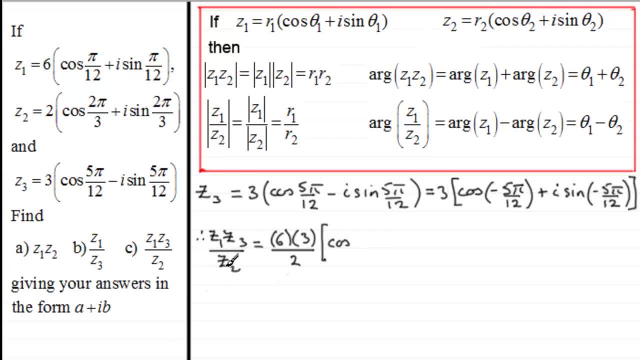 going to add the two arcs together and, dividing by Z 2, subtract the arc for Z 2. so in other words, we've got the cosine of: for Z 1 is going to be pi upon 12, and then we add this to the ARC for Z 3, which was 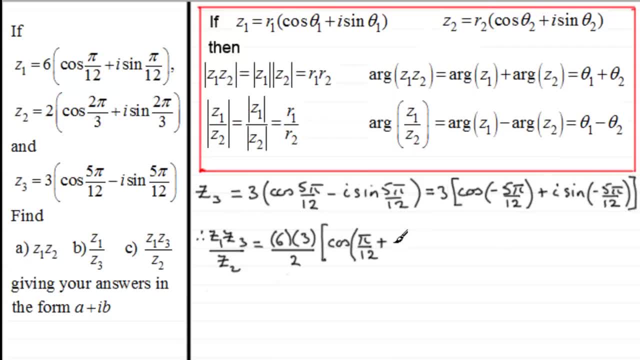 over here: minus 5 pi upon 12. nearly made a mistake there, so it's adding minus 5 pi upon 12, and then we're going to. We've got to subtract the arg for z2, and that was 2 pi upon 3, so minus 2 pi upon 3.. 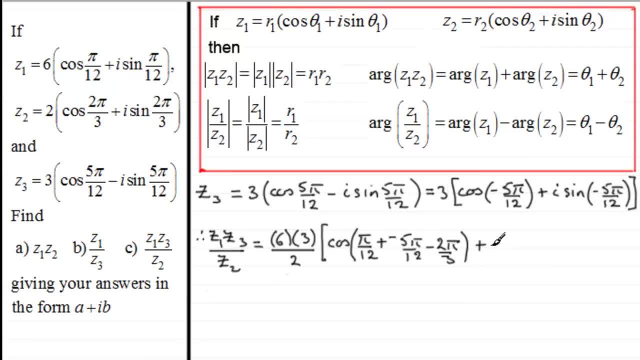 OK, hope you got that. And then plus i sine, and then we've got the same arg again as we had here: Pi upon 12, then plus minus 5, pi upon 12, minus 2 pi upon 3. OK, 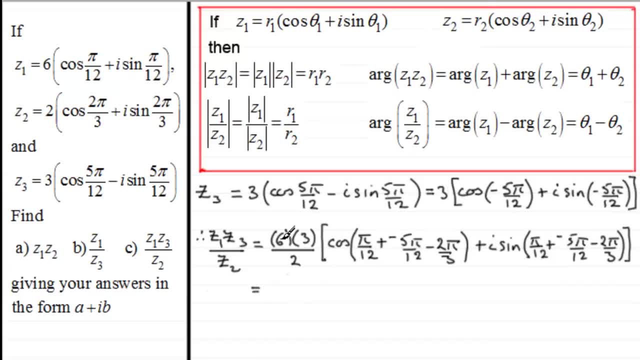 So if we clean this up, what we've got then is 18 divided by 2, which is clearly 9.. And then we've got the cosine cos for short, And if we do pi upon 12, minus 5, pi upon 12, minus 2, pi upon 3, that comes out to be minus pi. 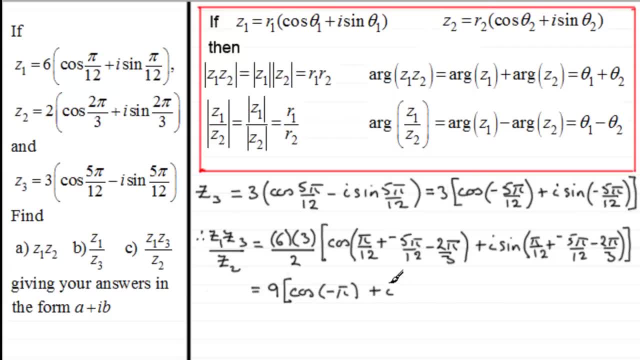 And then we've got plus i sine Also, So minus 5 pi by 2, which is equal to 0 of minus pi. And the cosine of minus pi: well, that's minus 1.. And the sine of minus pi: well, that's zero. 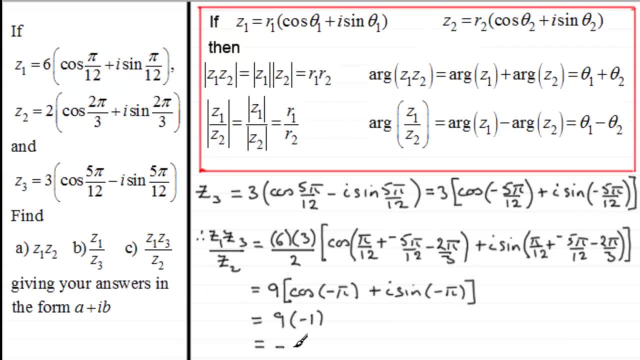 So you've just got a real value here 9 times minus 1, which is minus 9.. OK, So I hope that's given you an idea, across all three questions, to do questions similar to this okay. 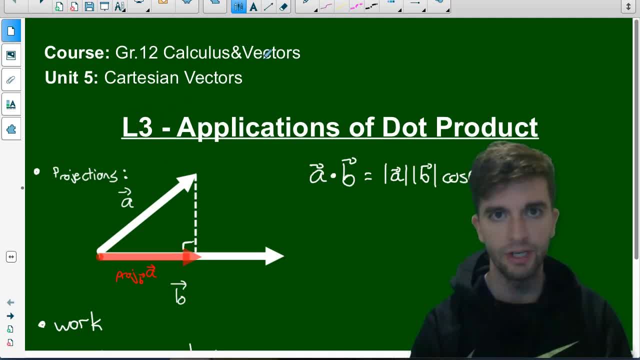 This is Lesson 3, Applications of Dot Product. This is from the Grade 12 Calculus and Vectors course, from the 5th Unit, Cartesian Vectors. So in the previous lesson we learned about the formula for dot product and in this lesson we're going to use our understanding of dot product.